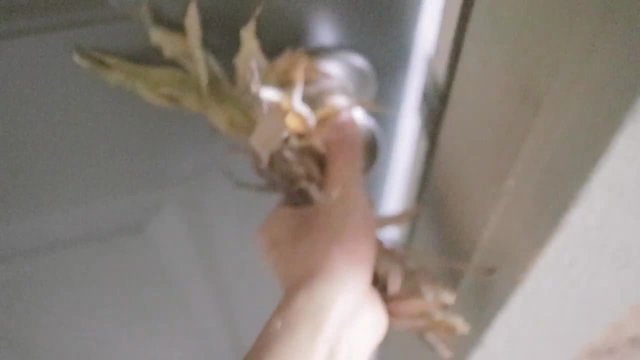 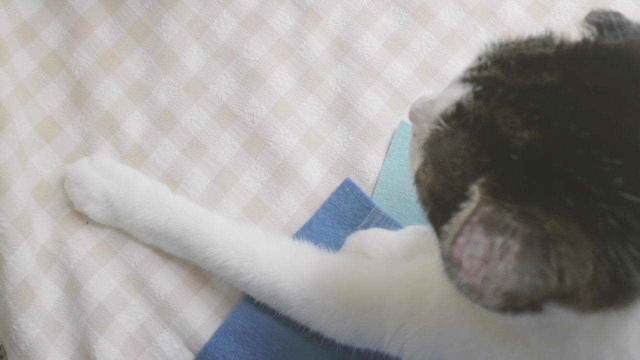 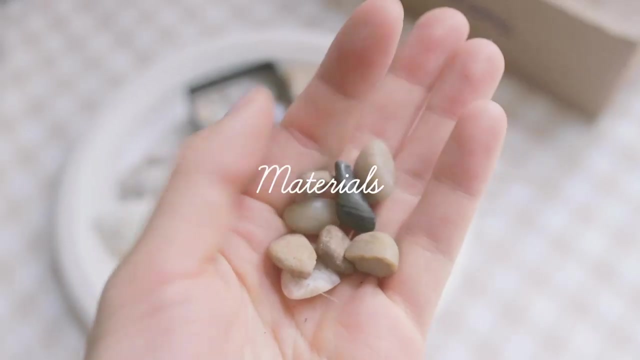 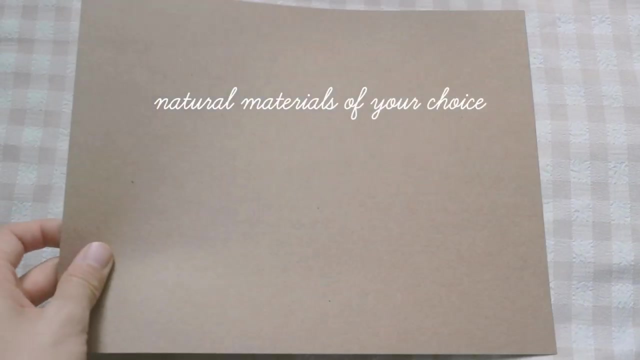 from the stores, which can include pine cones, pebbles, moss, cinnamon sticks and shells. I picked up some things from outside my home and used what I already had at home. What you need are some natural materials, a box, a paper or cardboard. I also included some felt. 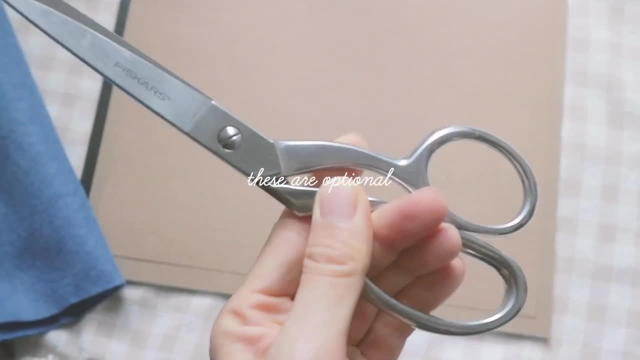 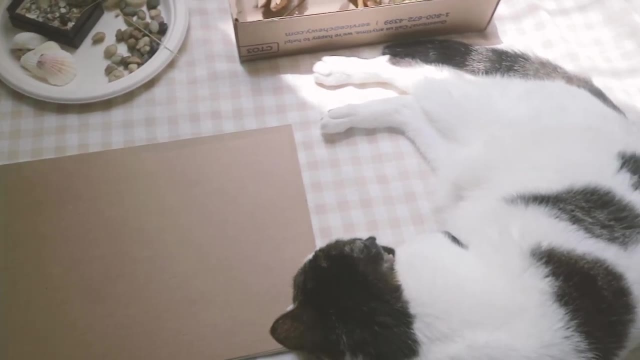 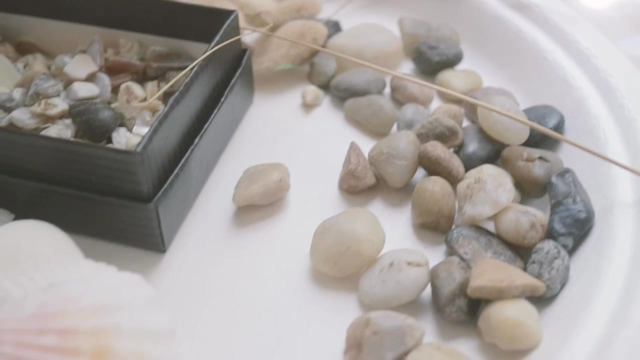 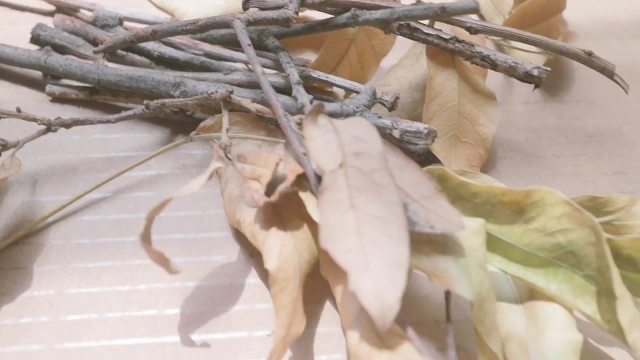 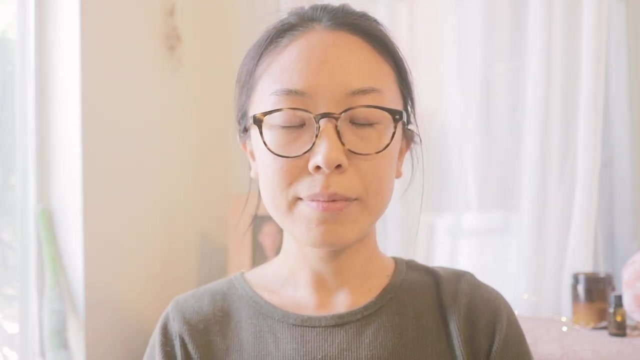 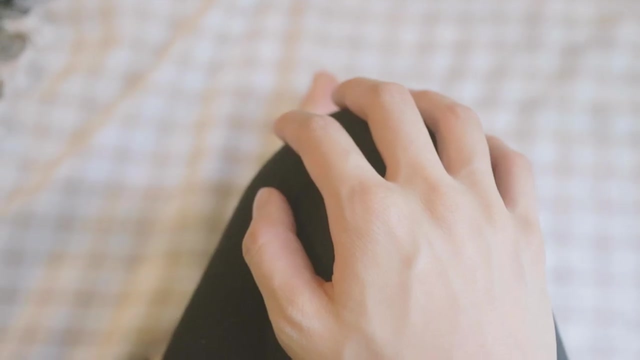 and scissors, and you will need a glue. Before making art, invite mindfulness and gently place your attention on your breathing and your body. When you think of nature, what feelings or thoughts come to mind? Also, set an intention today to make art without judgment and instead enjoy the creative process. 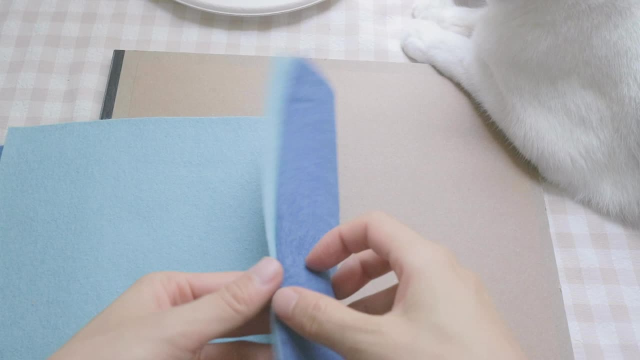 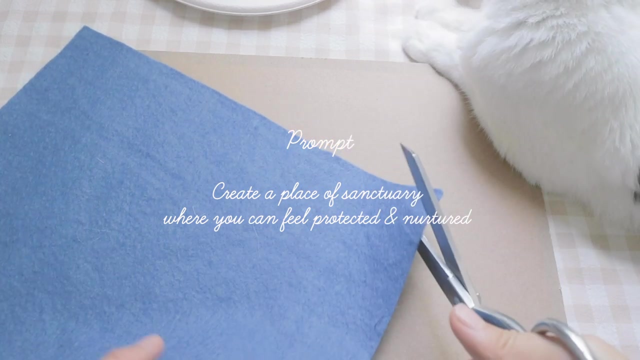 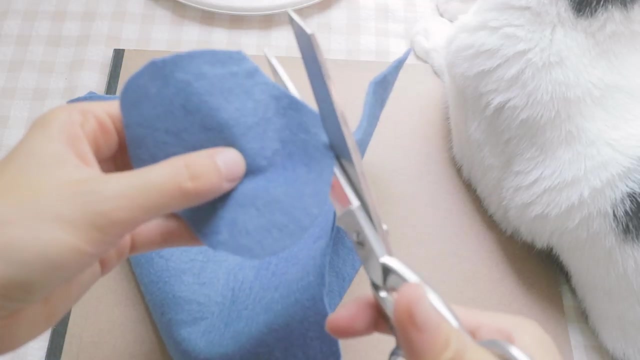 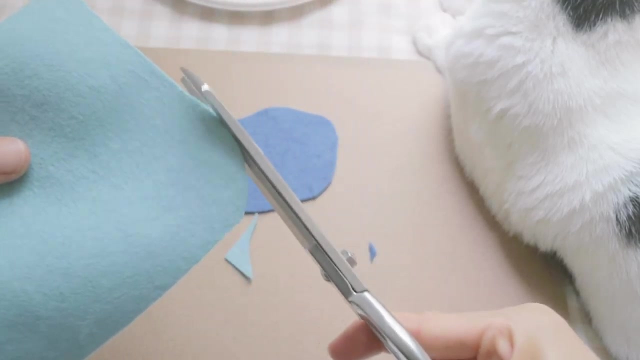 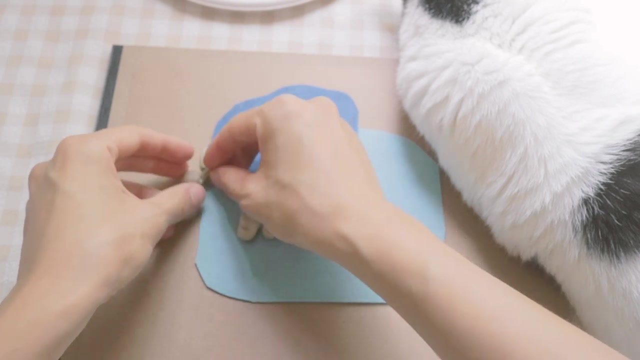 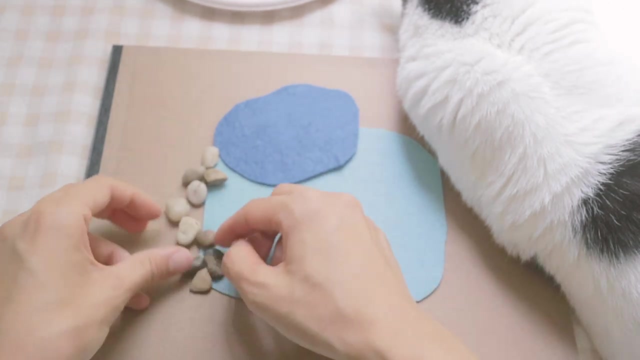 The prompt is to create a place of sanctuary where you can feel protected and nurtured. Nature has a way of giving us what we need to heal and feel nurtured and it really helps us to go outside, make that connection with nature and fill our soul up and become more active and use our resources around us. 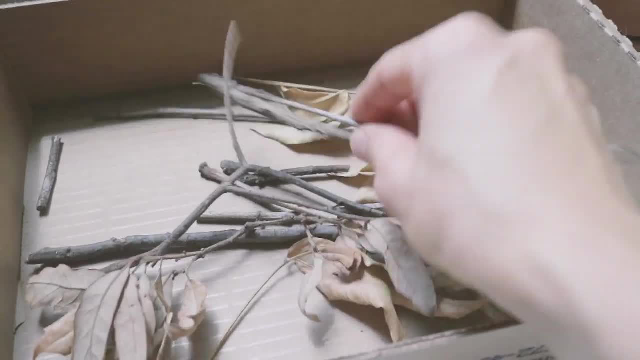 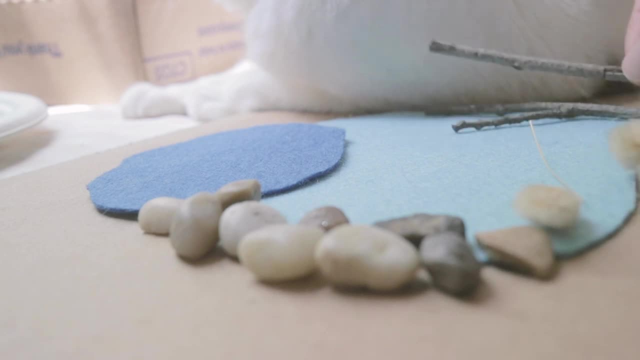 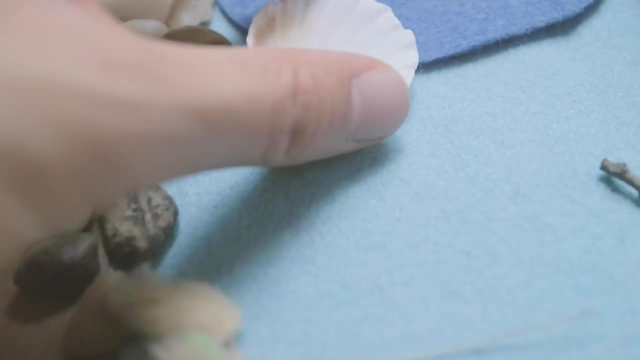 I think that using natural materials also lets us release our perfectionistic tendencies, because nature itself is imperfect and the material itself is imperfect, and the material itself is imperfect. The materials that we have are imperfect, so it's a wonderful way to use imperfect materials.